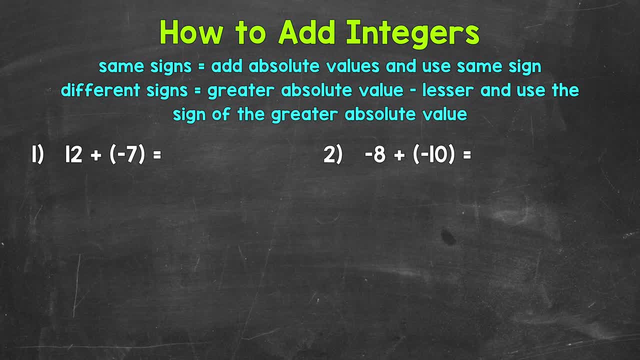 We will go through two ways for each of our examples. Let's jump into number one, where we have 12 plus negative 7.. We'll start this problem by taking a look at the signs. We have a positive 12 and a negative 7, so we have different signs, a positive and a negative. 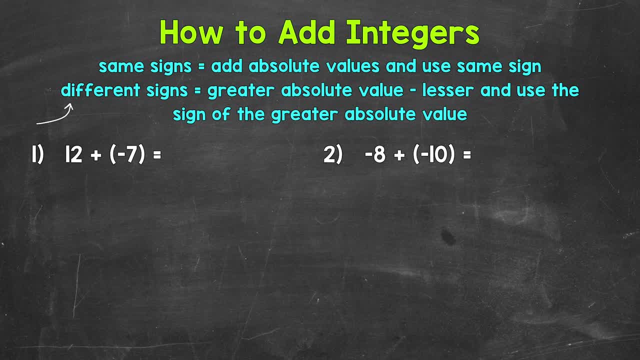 Since we have different signs, we are going to take the greater absolute value and subtract the lesser. Our answer will take the sign of the greater absolute value. Let's start by writing the absolute value of both 12 and negative 7.. And remember, absolute value is the distance a number is from 0.. 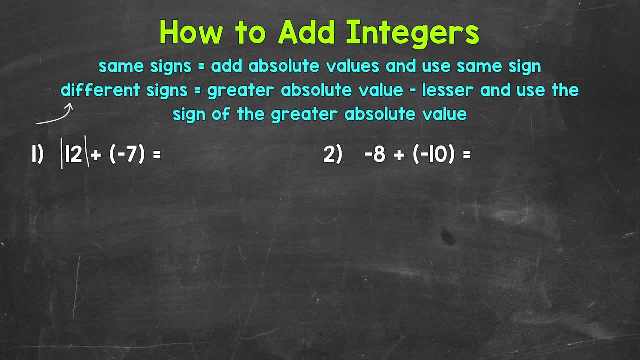 The absolute value of 12 is 12.. The absolute value of negative 7 is 7.. Now we take the greater absolute value and subtract the lesser. These are already in order, so we can subtract. The larger absolute value comes second. 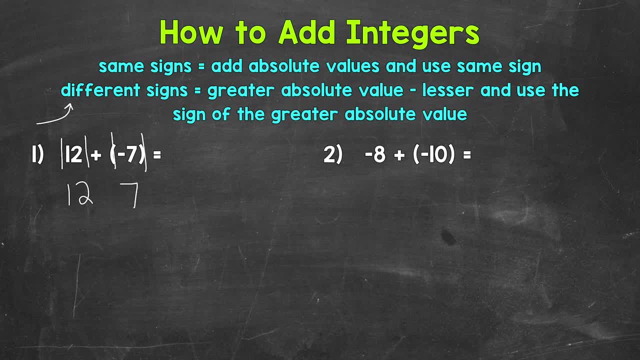 You can always switch the order to find the difference, if need be. Let's subtract, So 12 minus 7 is 5.. Now we need to determine if our answer is going to be positive or negative. So we need to take a look at the larger absolute value, which is this: 12.. 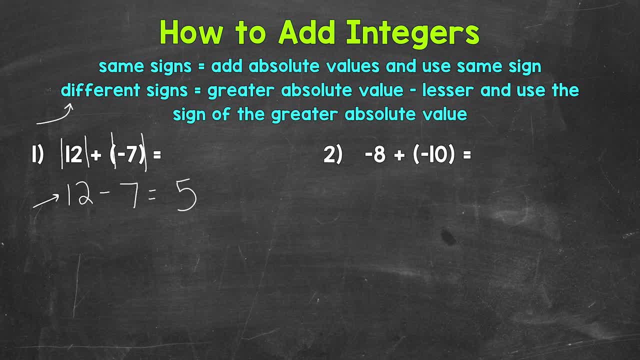 So we take the sign of the larger absolute value From the original problem, so the larger absolute value is 12.. Let's take a look at the 12 in the original problem and that 12 is positive. That means our answer is going to be positive. 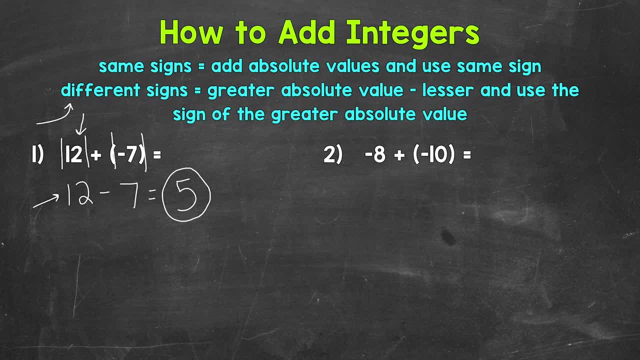 So our final answer? a positive 5.. So a quick recap here. Basically, we forgot about any negatives because we were working with absolute values. We then found the difference between the absolute values, And then we found the difference between the absolute values and the negative values. 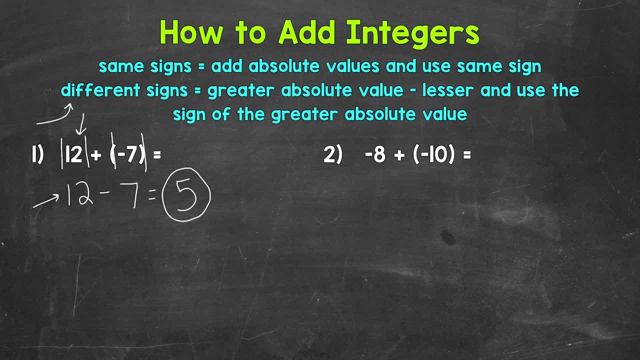 And the answer takes the sign of the greater absolute value from the original problem. Now let's think through this another way, And this way is going to be more of a mental math approach, Just basically thinking about what's going on in this problem. 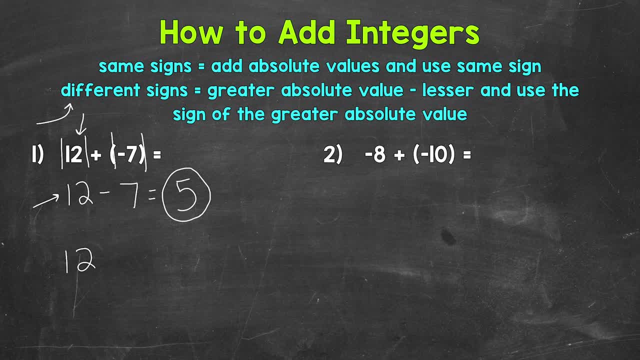 So let me rewrite 12 plus negative 7 here. So our original problem. So we are starting at a positive 12 and we are adding a negative 7 by adding a negative, by adding that negative 7.. We are decreasing in value by 7 from that 12.. 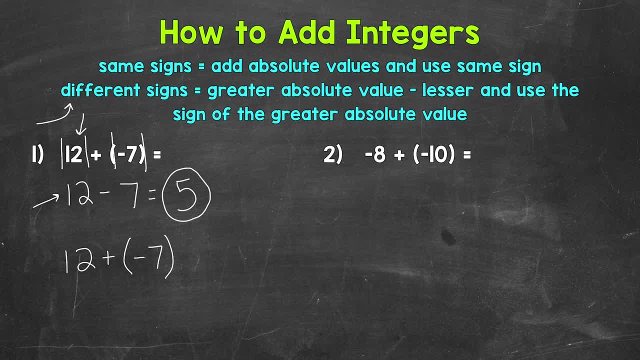 We can basically think of this as 12 minus 7, or 12 take away 7. that gives us our answer of 5.. So 12 plus negative 7. We are decreasing that 12 by a value of 7. So we get a positive. 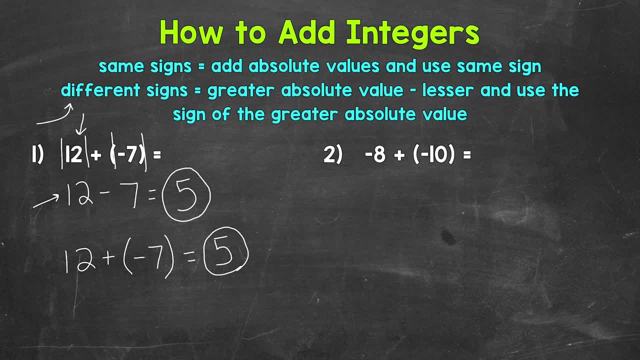 5.. So again, we started at a positive 12.. Always think about where you are starting and where you are going from that starting point. So we are adding a negative 7, which is decreasing our 12 in value by 7, and we end up with 5.. 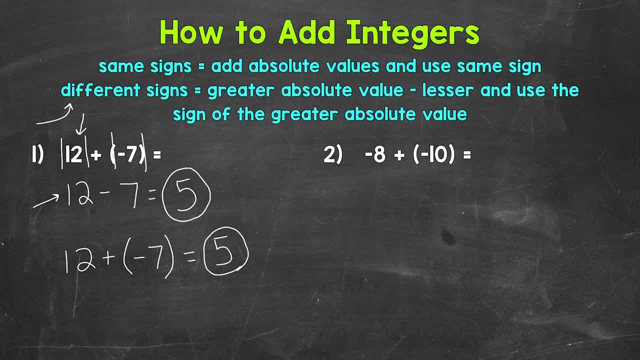 Let's move on to number 2, where we have negative 8 plus negative 10.. Here we have two negatives, So the same signs. So we are going to add the absolute values and use the same sign. So let's start by taking a look at the absolute value of negative 8 and negative 10.. 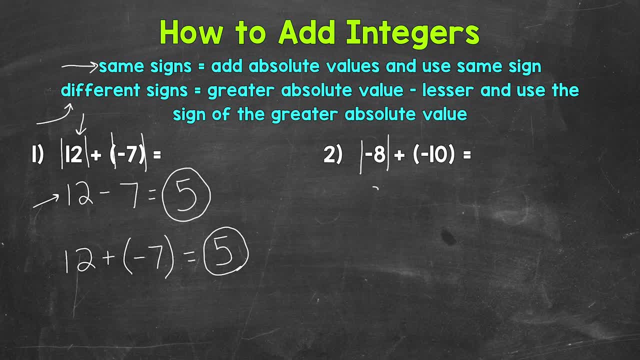 The absolute value of negative 8 is 8.. Plus the absolute value of negative 10, which is 10.. Now we add those absolute values because again we have the same signs: 8 plus 10 is 18.. We use the same sign from the original problem, which those are negatives there. 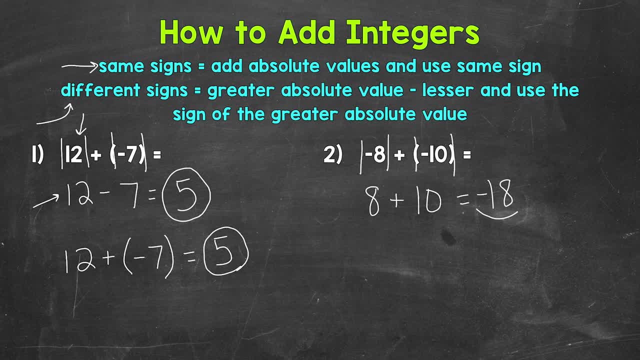 So our answer is negative. Final answer: negative 18.. Now, if we were to think through this, we can think that we are starting at negative 8.. So let me rewrite here: Negative 8 plus negative 10.. So again starting at negative 8.. 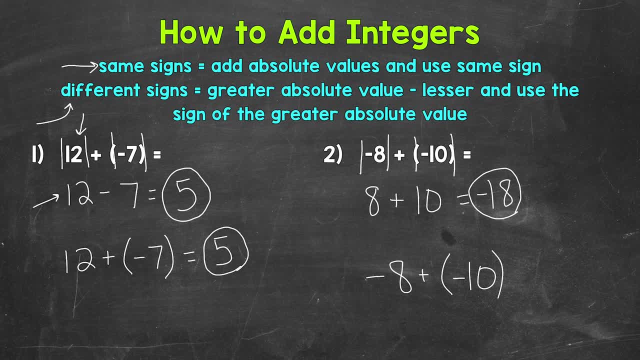 And we are adding a negative 10. So that means we are decreasing in value by 10. That leaves us at negative 18.. Like I mentioned earlier, think about your starting point. So the number you are starting with: We have a negative 8..